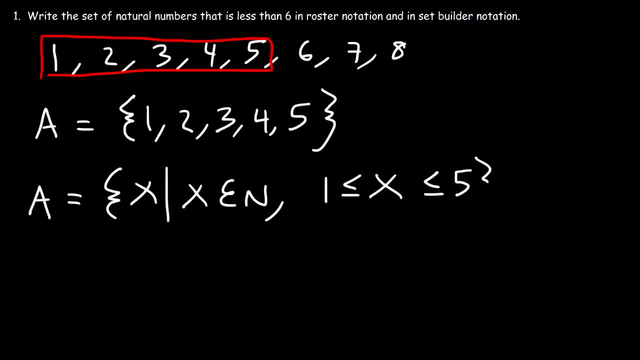 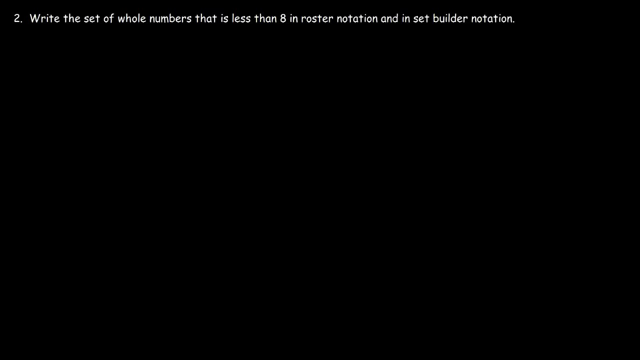 less than or equal to 5.. So that's how we can describe this set using set-building notation. So let's go ahead and work on some more examples. Number two: write the set-building notation in roster notation. We write the set of whole numbers that is less than 8 in roster notation and in set-building. 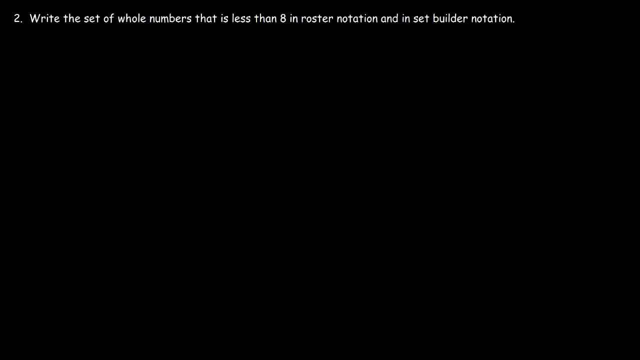 notation. So whole numbers are natural numbers, but they also include 0. These are all whole numbers, And we only want it less than 8. So we need to stop at 7.. So that's the list, And let's use B as heart. 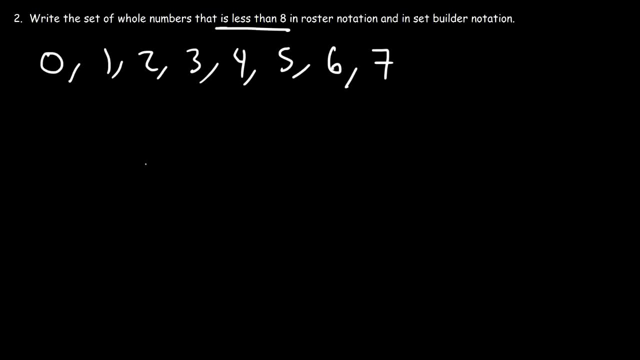 Let's focus on Dakotas, dominant and the added unit as the name of the set. So in Rasta notation, set B contains the elements zero, one, two, three, all the way up to seven. So in Rasta notation. 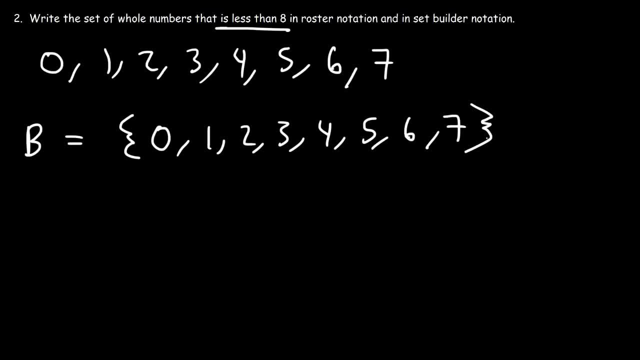 you just simply need to list the elements in the set. Now let's describe it using set building notation. So we could say that B is the set of all X, such that X is a whole number. I'm gonna use a W to represent a whole number. 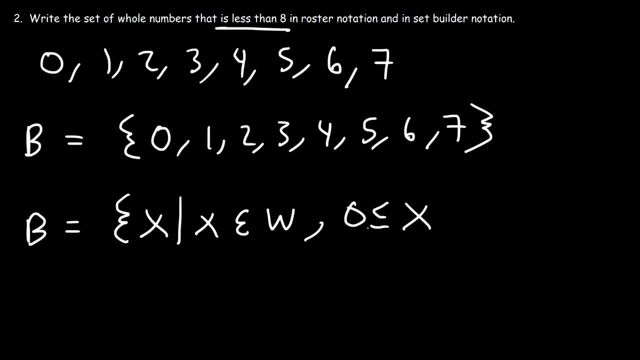 And also X is equal to or greater than zero, but it's less than eight, as we have it in the beginning of the problem. Now I could also say that X is equal to or greater than zero, but it's also less than or equal to seven. 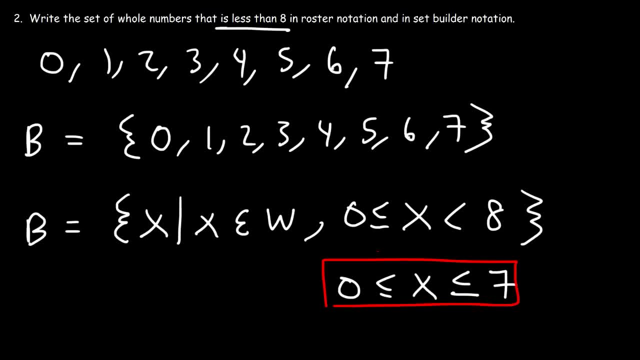 So both of these inequalities, or compound inequalities, they will describe this set of numbers, So you can use this one or you can use that one, doesn't matter. However, you do need to say that X is a whole number. Number three: write the set of integers. 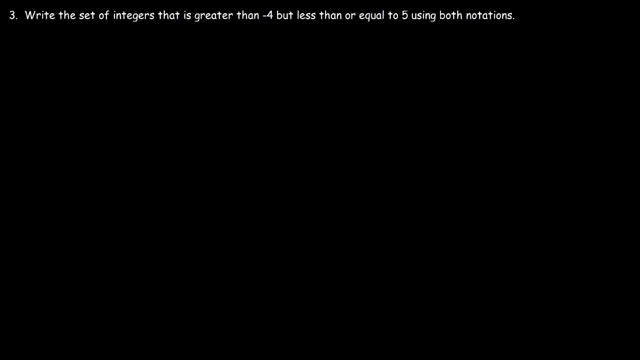 that is greater than negative four, but less than or equal to five, using both notations. So integers can be positive or negative and they include zero. Now the integer that is greater than negative four is negative three. And then we have negative two, negative one, zero one, two. 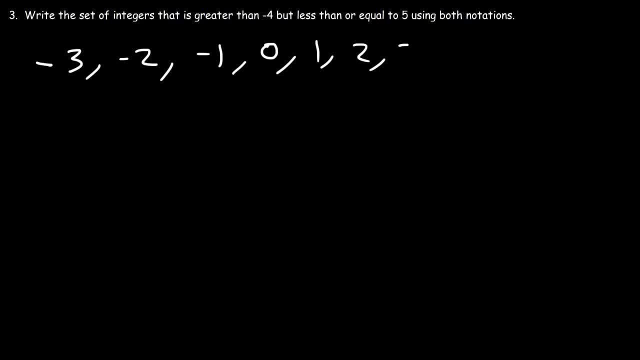 Now it has to be less than or equal to five, So it includes five. So that's the list of numbers that we have. So let's use sets Set C. So in ROSA notation, set C will contain these elements. Now what about in set builder notation? 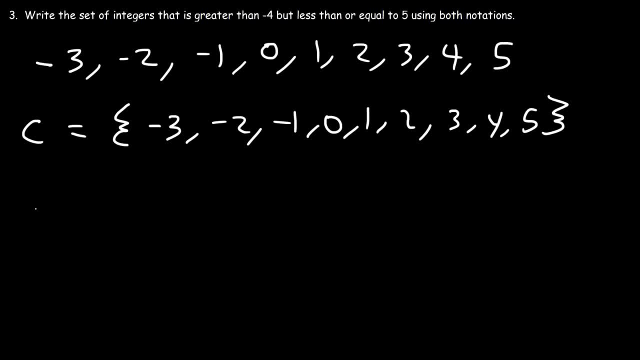 How can we describe it? So we could say that set C or C is the set of all Xs, such that X is an integer. I'm going to use I to describe integer And it's between negative three and five. Or I could say that it's greater than negative four. 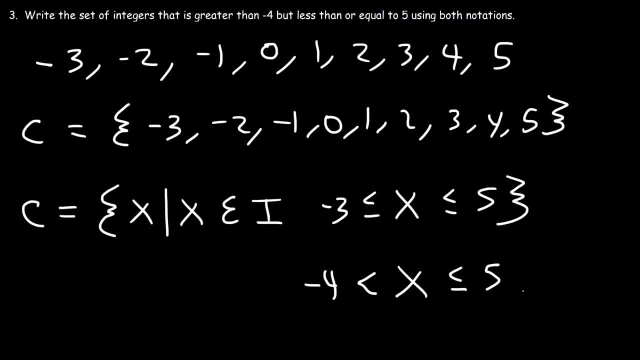 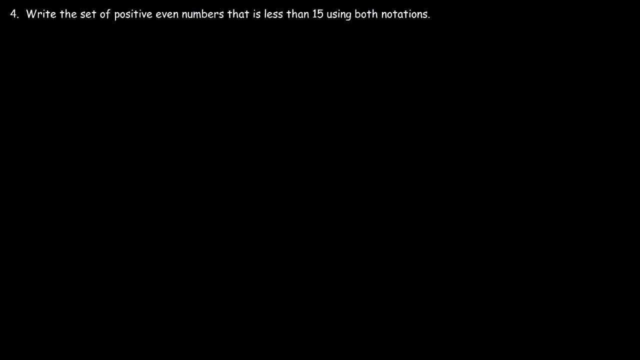 but it's less than or equal to five, So both ways work. So now you know how to describe a set using set builder notation, or using, you know, set builder, Or using the ROSA method Number four. Write the set of positive even numbers. 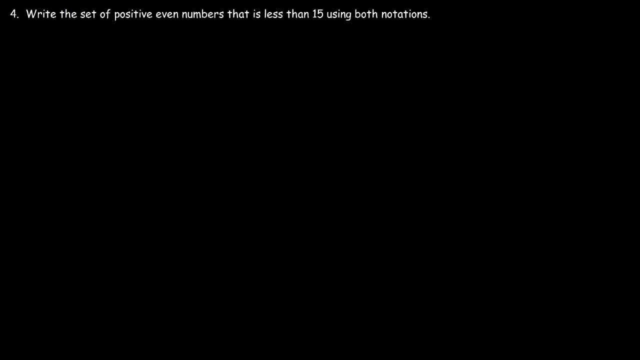 that is less than 15 using both notations. So let's use D as the name of the set And let's start with the ROSA notation. So even numbers. they have to be positive. Two is a positive even number. Four, six, eight, 10.. 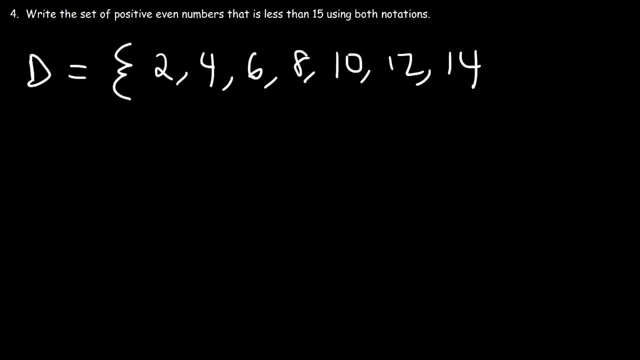 And we're going to stop at 14, because it has to be less than 15.. And 15 is an odd number. So this is the list in ROSA notation. Now let's describe set D using set builder notation Now, instead of using the letter X, 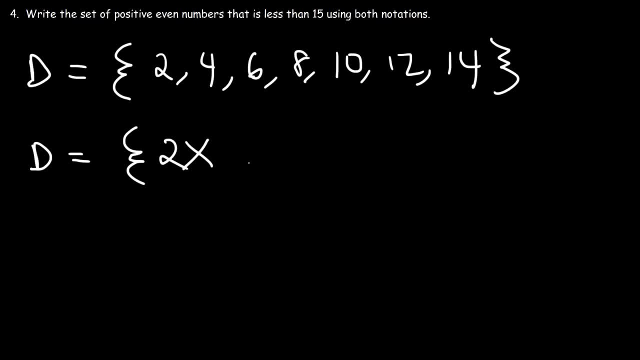 I'm going to use two X, because the numbers differ by two. Now I'm still going to say that X is, in this case we can use, a natural number. All of these are natural numbers And X has to be between one and seven. 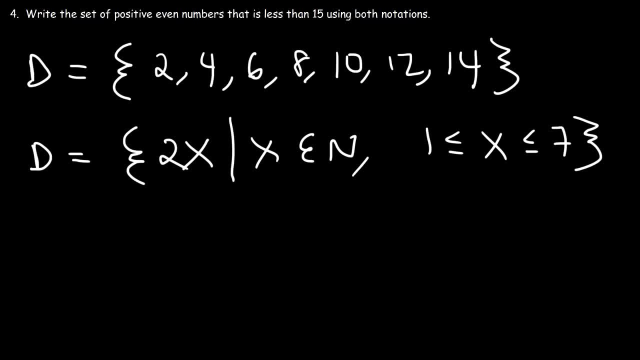 Now let's make sense of this: When X is one, two X will have a value of two. Two times one is two, And when X is seven, two times seven will give us the value of 14.. And so, from one to seven. 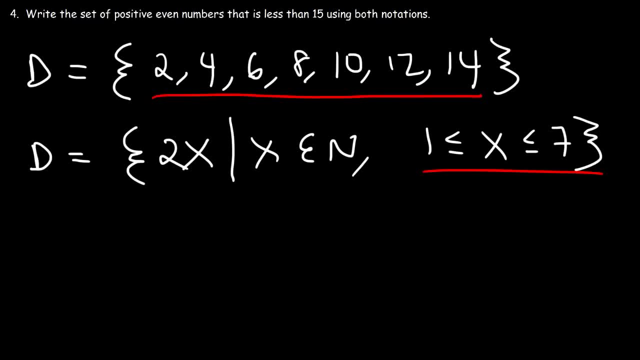 we'll get the numbers two, four, six, eight, 10,, 12,, 14.. So when X is two, two X or two times two will be four. When X is three, two times three will give us six. 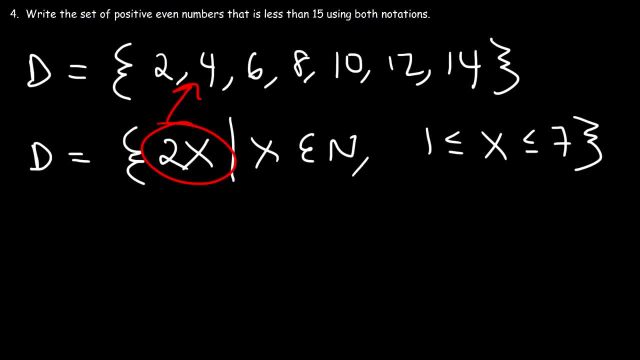 When X is four, two times four will give us eight, and so forth, And so that's it for this problem. So that's how you can describe this set using the ROSA method and the set builder, notation Number five: write the set of odd numbers. 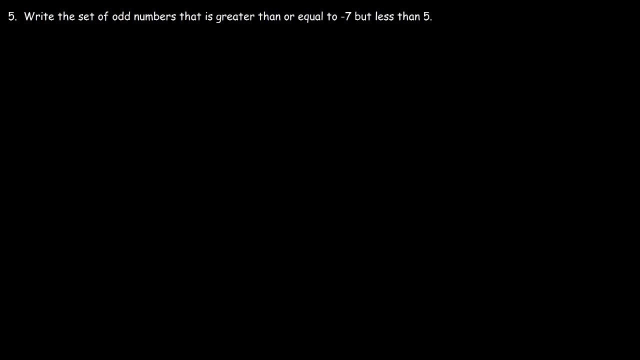 that is greater than or equal to negative seven, but less than five. So let's use the letter G And let's start with ROSA notation Now. it's greater than or equal to negative seven, And negative seven is simply a negative odd number. 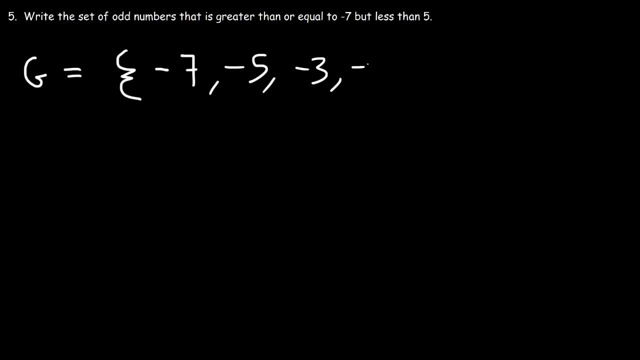 Negative. five is also an odd number. And then we have negative three, negative one, negative two. negative one, negative three, negative one. Now we cannot include five. It has to be less than five, It's not equal to it. 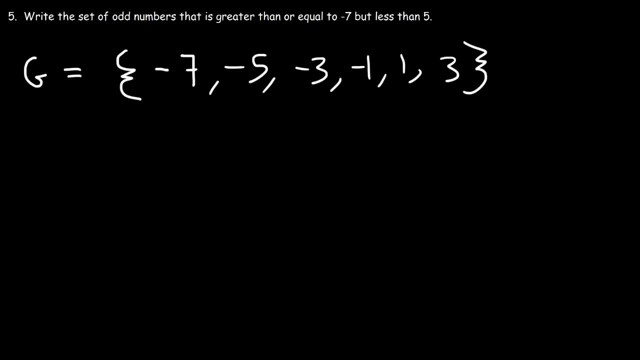 So we need to stop at three. So that's set G in ROSA notation. Now let's describe set G in set builder notation. So once again, we simply need to use two X as opposed to X, But for odd numbers we're gonna add one to it. 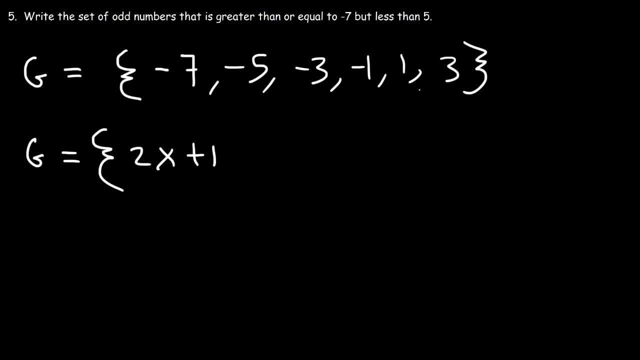 So we're gonna say two X plus one, because if we simply use 2x, we're going to get even numbers. but if you want odd numbers, use 2x plus 1, because the number still differs by 2.. Now we're going to. 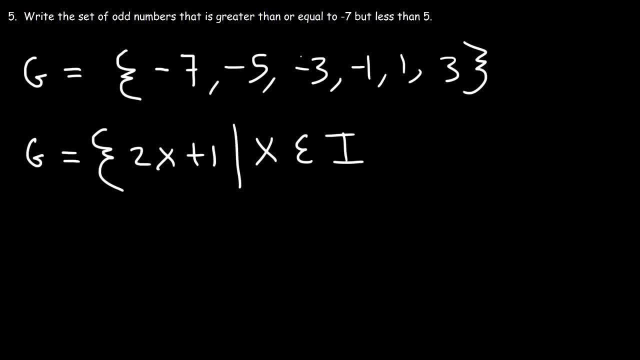 say that x is an integer, because these are not natural numbers, they're integers- and at the same time, we need to say x is between two numbers. Now, which two numbers should we use To find the two numbers? what we're going to do is set. 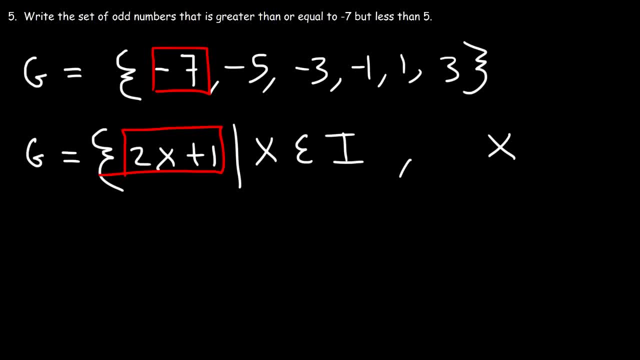 negative 7 equal to 2x plus 1.. So let's start by doing that first. So I'm going to subtract both sides by 1. Negative 7 minus 1 is negative 8. And that's equal to 2x, and then divide by 2. Negative 8 divided by 2 is 4.. So x. 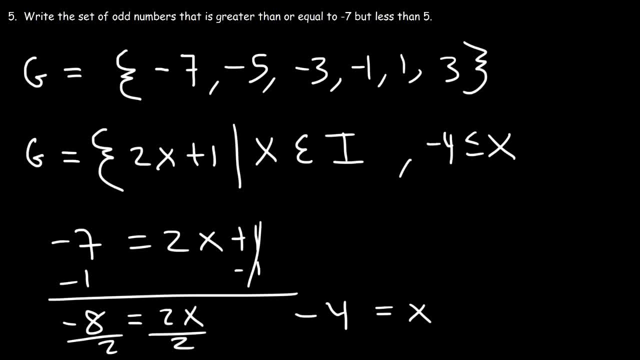 has to be equal to or greater than negative 4.. That's the first number. Now let's find the second number. So we're going to set 2x plus 1, equal to the last number of the set, That's 3.. 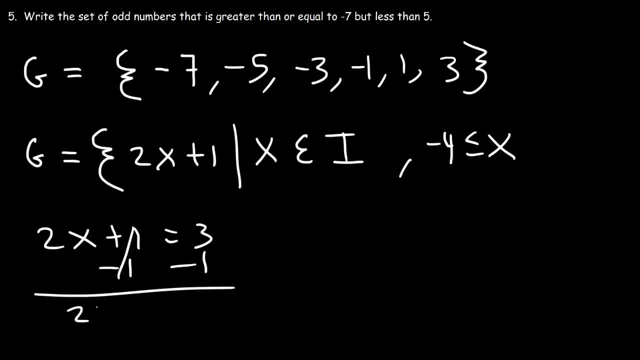 And so let's subtract both sides by 1.. So we're going to subtract both sides by 1.. And so let's subtract both sides by 1.. 3 minus 1 is 2.. And then, if we divide both sides by 2, x is 1.. So x has to be. 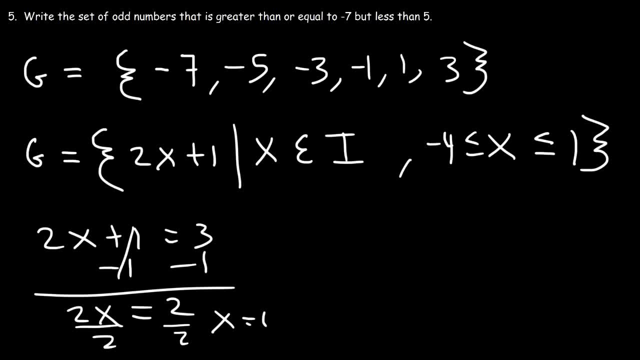 between negative 4 and 1.. So if we were to plug in negative 4 into this, 2 times negative 4 is negative 8 plus 1. That will give us negative 7.. If we plug in the next number in this list, that's negative 3.. 2 times negative 3 is. 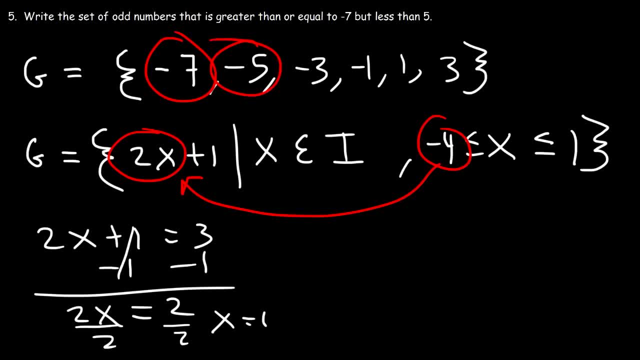 negative 6 plus 1. That will give us negative 5.. And so this equation will describe this set of numbers when these numbers are plugged in into that expression. So, for example, if I plug in, x equals 0,, 2 times 0 is 0 plus. 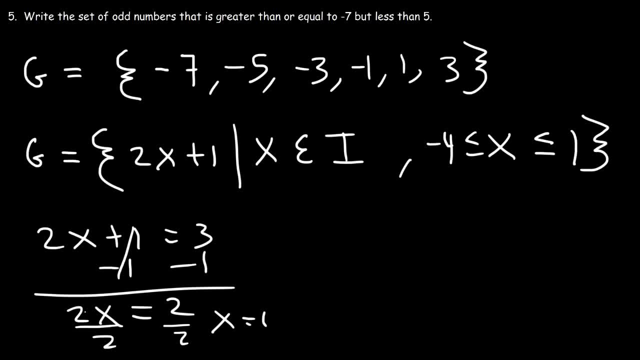 1. That will give me this number. If I plug in negative 1 for x, 2 times negative, 1 is negative 2 plus 1.. That will give me negative 1.. And if I plug in the last one, positive 1, 2 times 1, is 2 plus 1.. That will give me the last number, positive 3.. 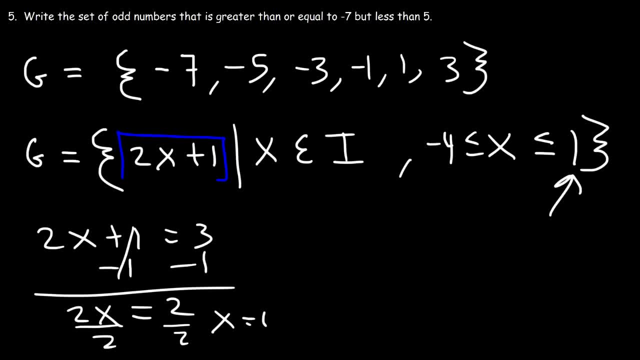 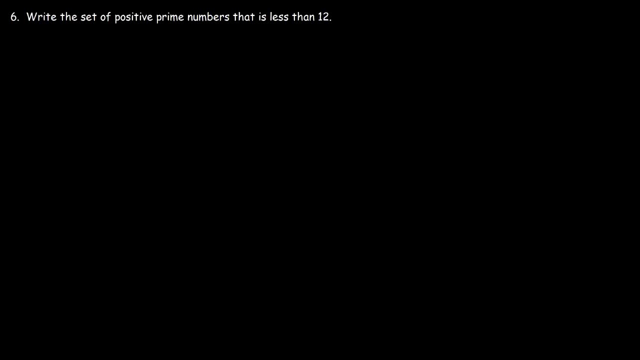 And so you want to make sure that you have the right algebraic expression plus the values of x that go into it. that will produce an output that gives you this, these set of numbers. And so that's it for number 5.. 6. Write the set of. 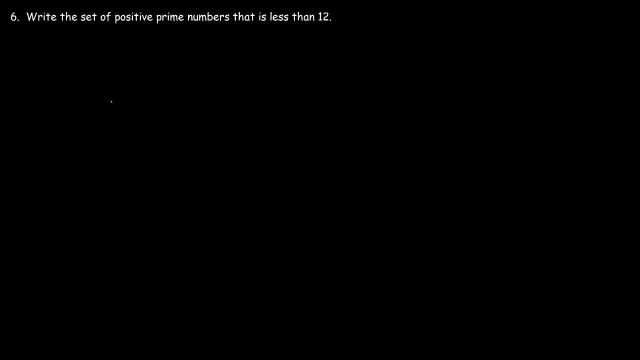 positive prime numbers that is less than 12.. So let's use k as the name of the set and let's do so in roster notation. So 1 is a prime number and it's positive 3, actually 2 is a prime number, 3 is a prime. 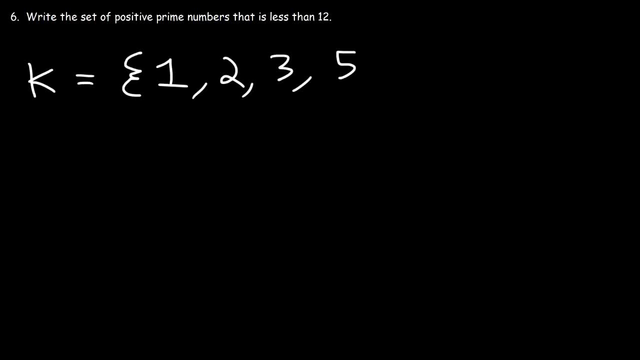 number 4 is not a prime number because 2 times 2 is 4.. 5 is a prime number. And then we have 7.. 9 is not a prime number because 3 times 3 is 9.. And for 10, 2 times 5 is 10.. 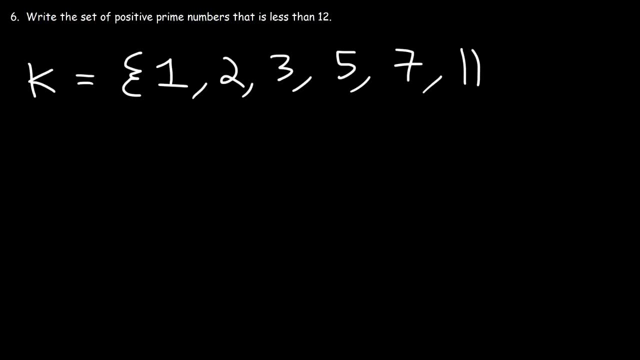 So that's not a prime number. 11 is a prime number, And we have to stop here. It has to be less than 12.. Now how can we describe it? using set building, So let's say that k is the set of all numbers, x. Now it's going to be hard to. 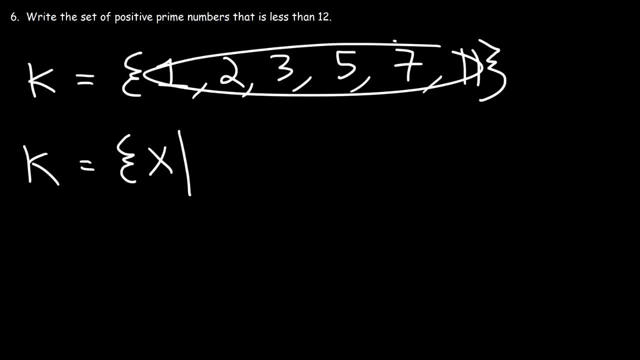 write an equation that will describe these numbers. So if it's difficult to write the equation, use words. So we could say x is a prime number And then we could say that x is between 1 and 11. Or we could say that x is less than 12.. Both 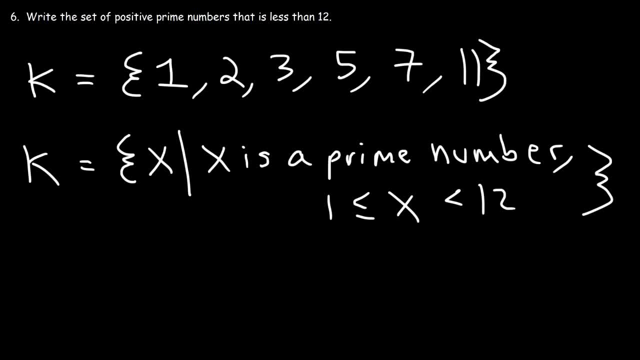 cases will be fine, And that's it. So, if you can't come up with a mathematical expression that will describe this pattern of numbers, use words, Keep it simple. So here is the last problem of this video: Write a set of positive perfect square numbers. 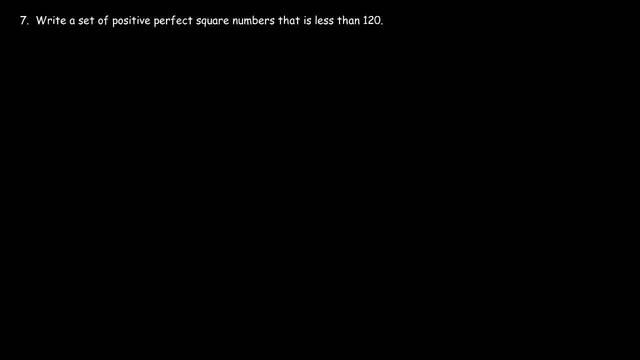 that is less than So let's use r as the name of the set. So 1 is a perfect square. 4 is a perfect square. 9 is a perfect square. The reason why 4 is a perfect square is because 2 times 2 is 4.. Or 2 squared is 4.. 3 squared is 9.. So 9 is. 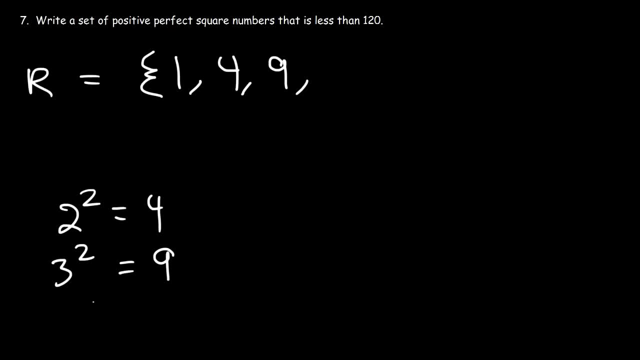 a perfect square. What is the next perfect square in the list? 4 times 4 is 16.. So that's the next perfect square: 5 squared is 25.. 6 squared is 36.. 7 squared is 49.. 8 squared is 64.. 9 squared: